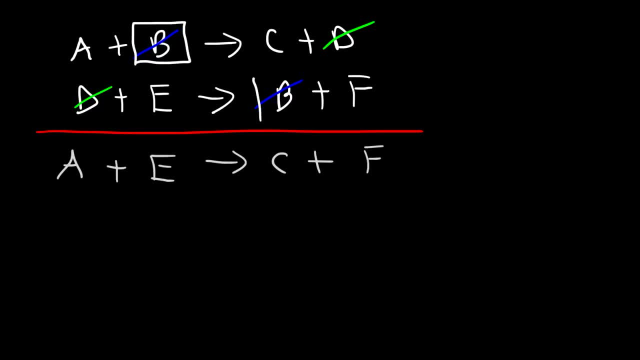 B is first produced and then I mean it's consumed first and then it's produced later. so B is the catalyst. it shows up on the left side first and then it shows up on the right side second. so make sure you understand that the catalyst is consumed first and then it's produced later on in the reaction. and that's how. 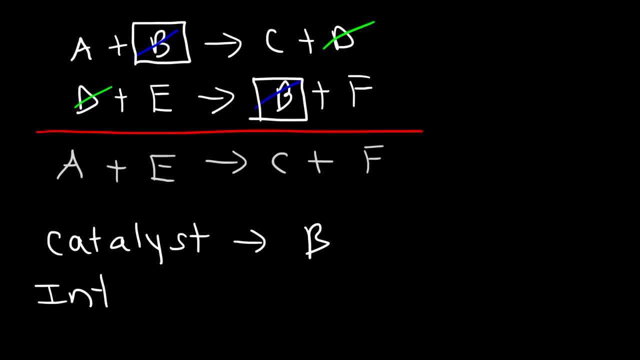 it's never used up. now the intermediate is the other stuff that was cancelled. the intermediate appears on the right side first and then shows up on the left side later. so D is the intermediate. it's produced first and then it's consumed later. the intermediate doesn't. 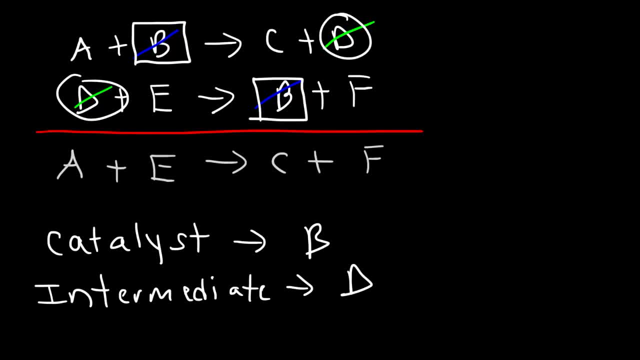 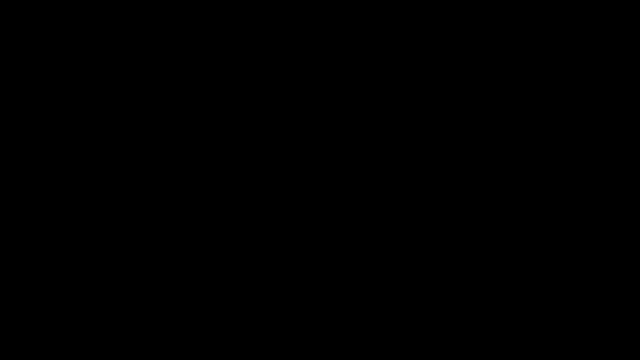 show up at the beginning or at the end of the reaction. it's somewhere in the middle of the reaction, so you really don't see it, but the catalyst is present at the beginning and at the end. now let's consider another example. A plus B yields C and D, and then C plus E produces F and G, and it's going to be a. 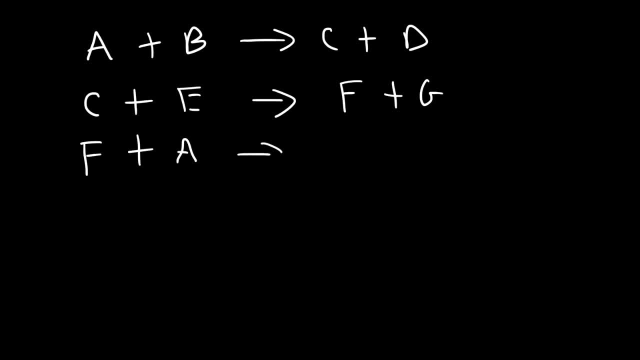 third step: F plus A makes B plus E. so, given these three steps, identify the intermediate and the catalyst. and just so you know, this gonna be two catalysts and two intermediates in this example. so let's find out what cancels. notice that B cancels. so is B a catalyst or is it an? 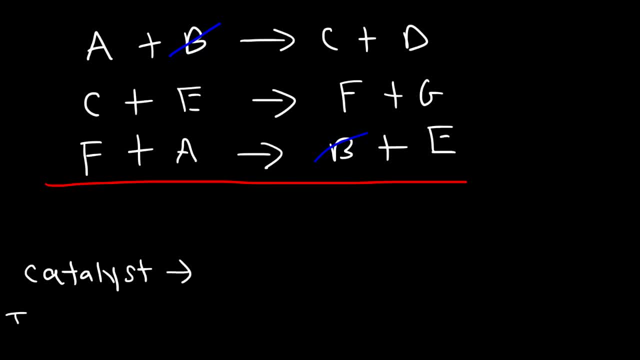 intermediate. what would you say now? B shows up on the left side first, and then later it shows up on the right side. It's consumed first and then it's produced later, which makes it a catalyst. Now let's look for the next species that cancels. 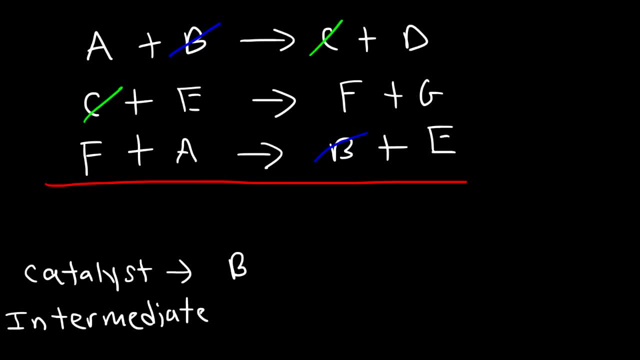 Notice that C cancels as well. C appears on the right side first and then shows up on the left side later, So it's produced first and then consumed later, which means C is an intermediate. Now, what else do you notice? Notice that E can be cancelled. 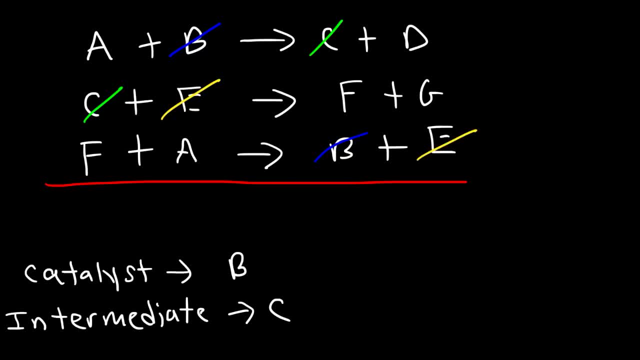 So E shows up on the left side first, and then it shows up later on the right side. So E is consumed first and then produced later. This means that E is a catalyst, just like B is a catalyst Now. next we have F.